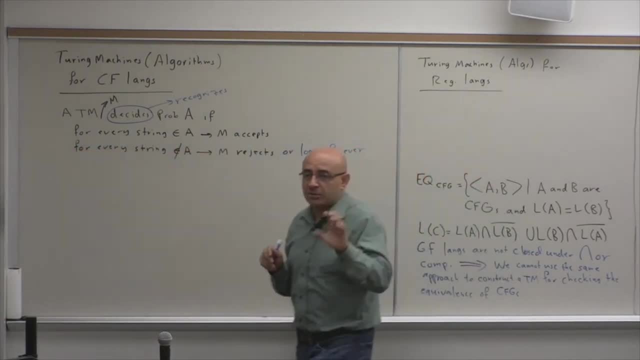 for deciding a language. If the string belongs to the language, it's going to accept. If it rejects, it's going to reject. If it doesn't belong to the language, it's going to reject. While recognizability means if a string belongs, it will accept, 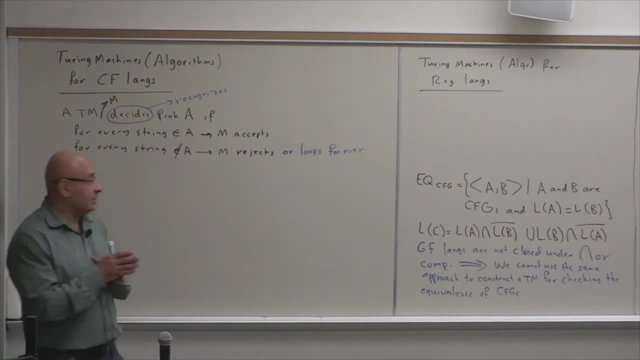 But if it doesn't belong, it will either reject or loop forever. So a recognizer may not terminate within finite time. A decider terminates within finite time. A decider makes a decision. A recognizer recognizes It, recognizes what belongs to the language. 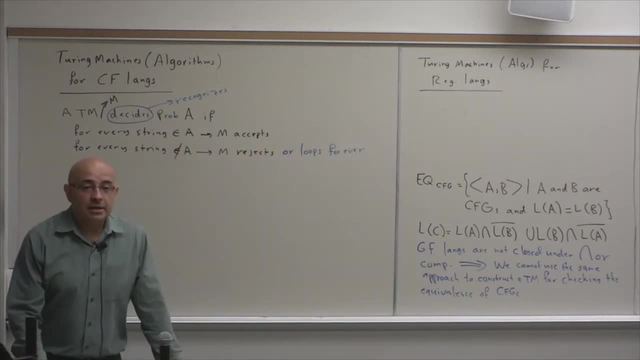 But if you give it something that doesn't belong to the language, it may loop forever. It may not give you an answer within finite time. Okay, Now, if what's interesting is that if a language, it's a string, If both the language and the complement. 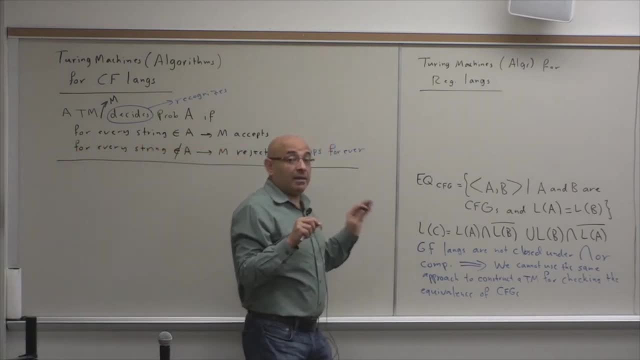 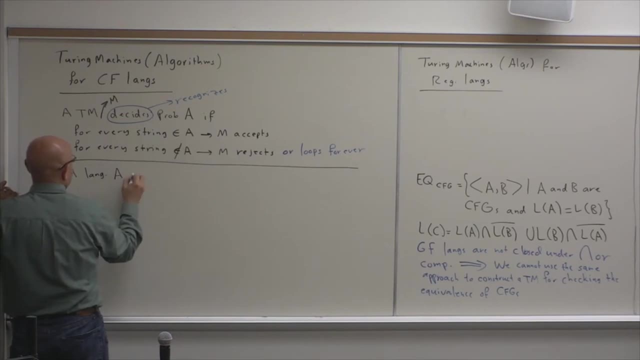 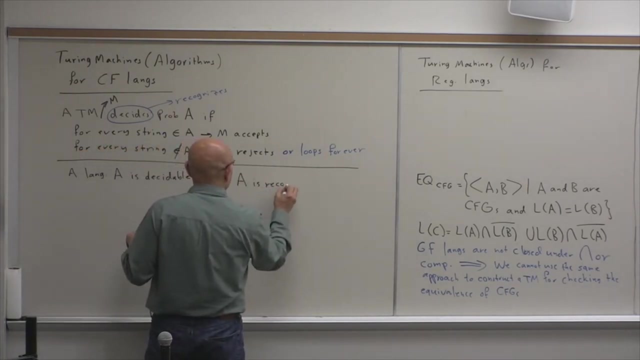 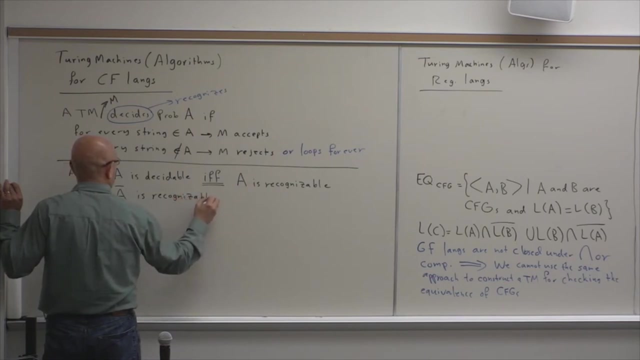 of the language are recognizable, then the language is decidable. So a language- A- is decidable if and only if, if and only if A is recognizable. Okay, So if A is recognizable and the complement of A is recognizable, The complement of A is recognizable- can also be phrased: 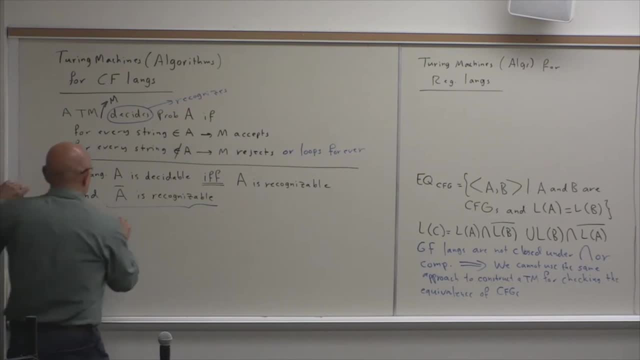 as A is co-recognizable. Excuse me. So when we say A is co-recognizable, it means that the complement of A is recognizable. Now, why is this the case? If you have, if you can, if you have a recognizer for the language? 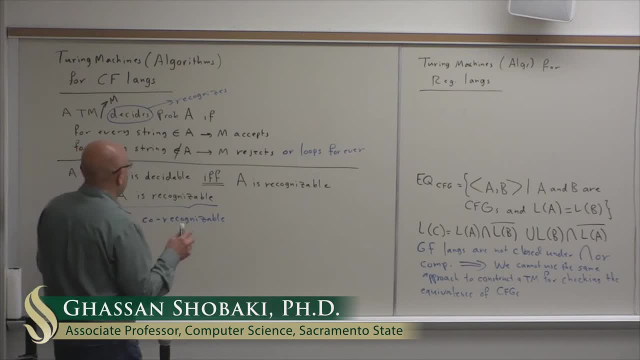 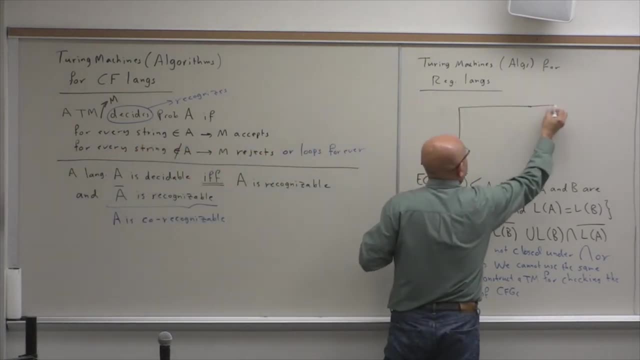 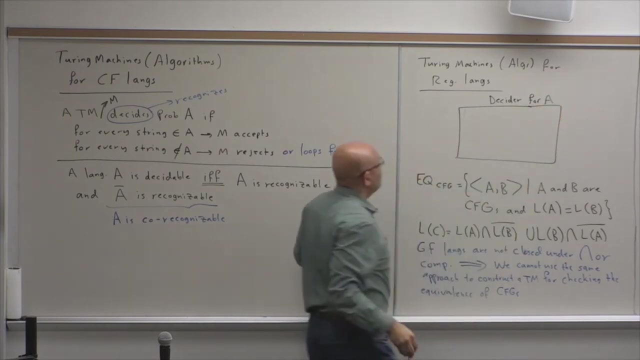 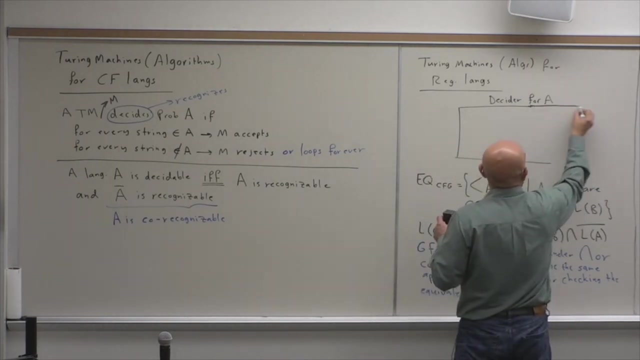 and a recognizer for the complement, then you can build a decider for the language. It's like a decider. Okay, So you can build a decider for the language. Decider for A would just run if you have a recognizer. 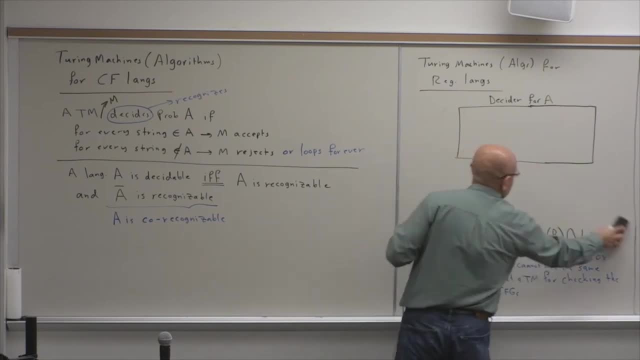 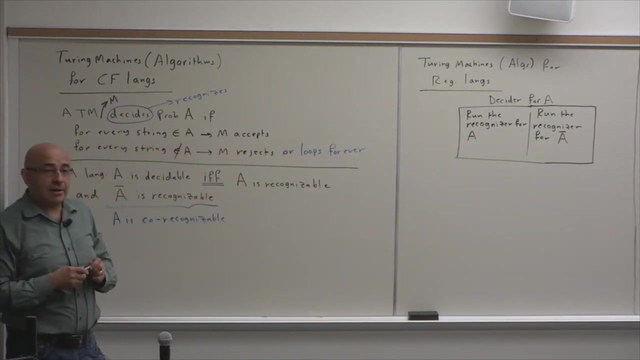 and a co-recognizer. you can build a decider. Okay, Run the recognizer, Recognizer, Recognizer, Recognizer, Recognizer, Recognizer For A and run the recognizer for A complement in parallel. So a decider for a language if you have a recognizer. 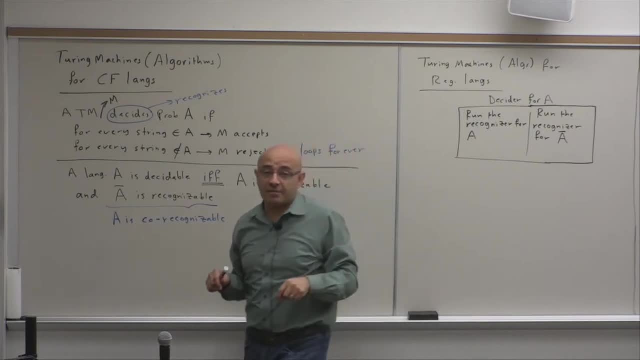 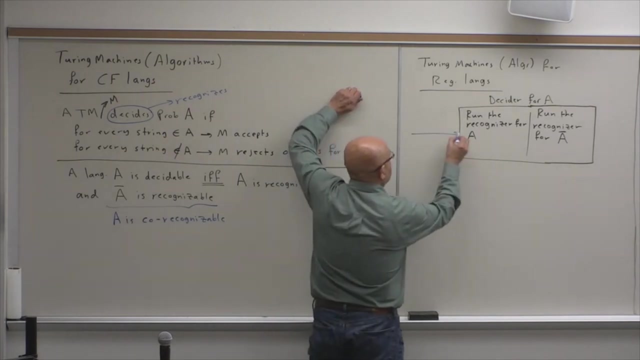 for the language and a recognizer for the complement of the language Right. You can decide the language. You are guaranteed to terminate within finite time. Why? Why is that Given any string? so if there is any input string, string W: 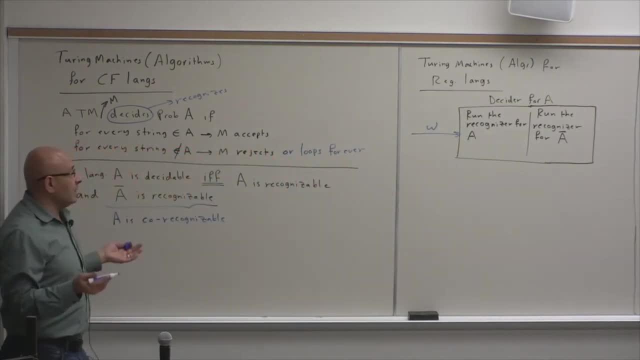 a string will either belong to the language or its complement, Because by definition, the complement of the language have all the strings that are in sigma star but are not in that language. So a string will get recognized by either this or this. 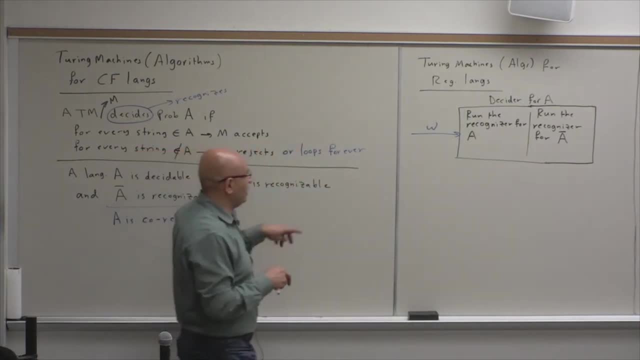 So we are guaranteed, if there is a recognizer for A and the recognizer for A complement, we are guaranteed that one of them is going to recognize W in finite time. Okay, So if you call this machine R, so if you have this, 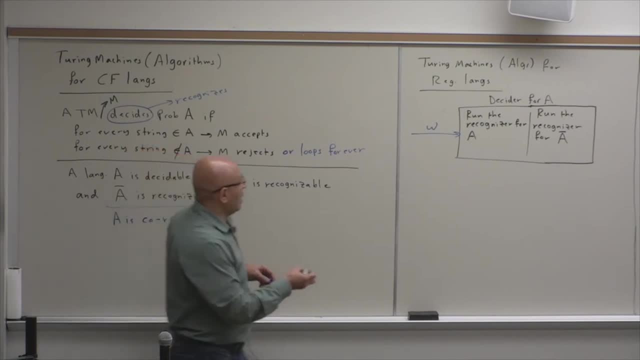 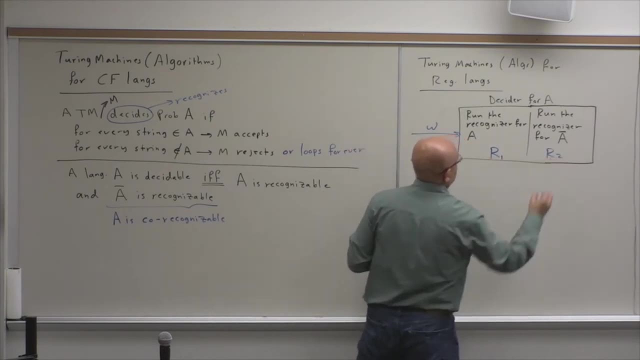 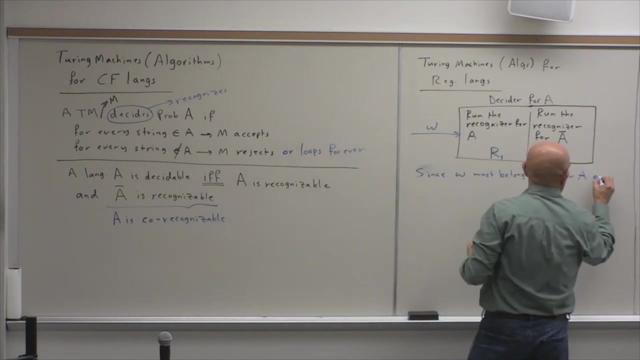 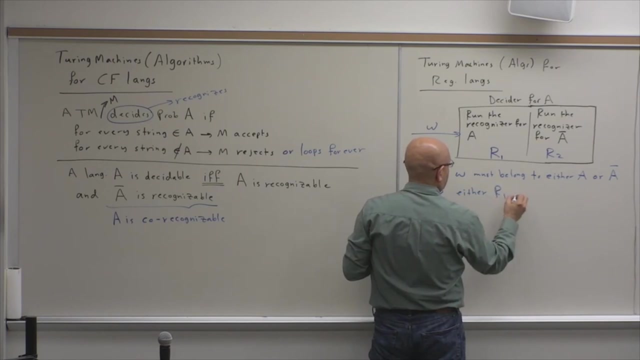 you will have to recognize it. You will have to recognize it, and R1 and this is R2, so either R1, since- okay, let's say, since W must belong to either A or A complement, then either R1 or R2 will recognize W. 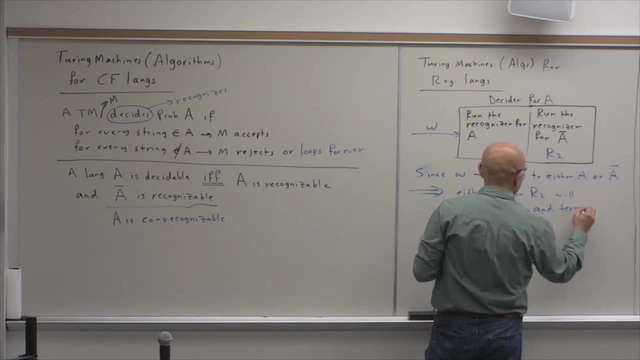 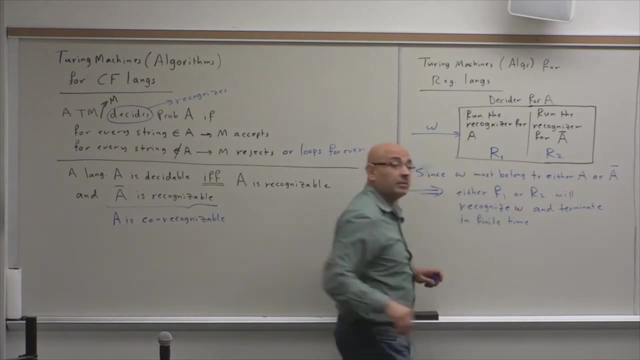 and terminate in finite time. One of them is going to recognize it, And when one of them recognizes it, you make a decision. So if R1 recognizes it, you accept, If R2 recognizes it, you reject. So this is the you know the algorithm. 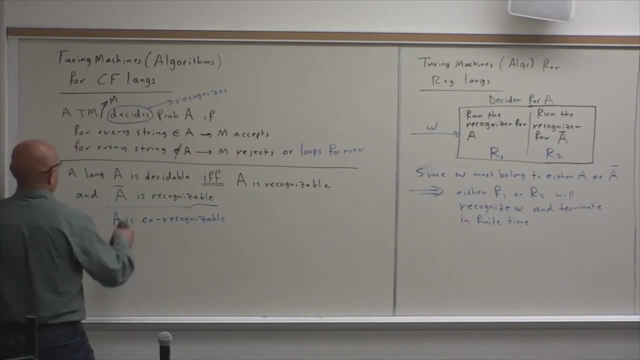 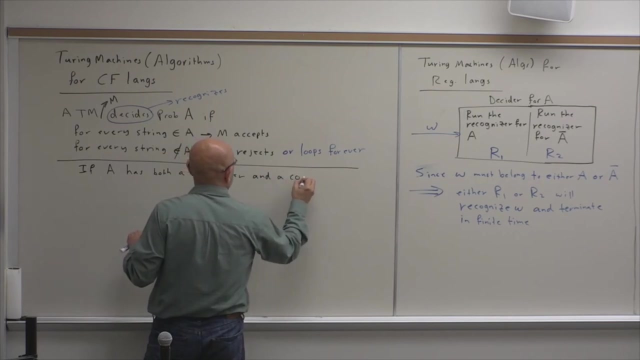 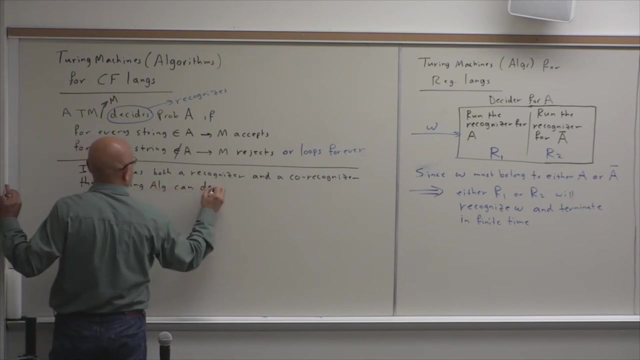 for building a decider using two recognizers. So if a language, if A, has both a recognizer and a decider, then A has both recognizers And a corecognizer. the following algorithm can decide A. So algorithm or Turing machine M run. 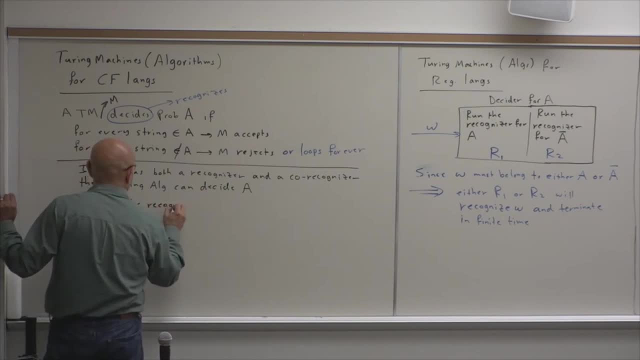 The recognizer R1 for A And the recognizer for the recognizer R2 for A complement, And in this case, of course, we must use this, So we need to have the two promising that one of them is going to accept If A is going to accept the other.